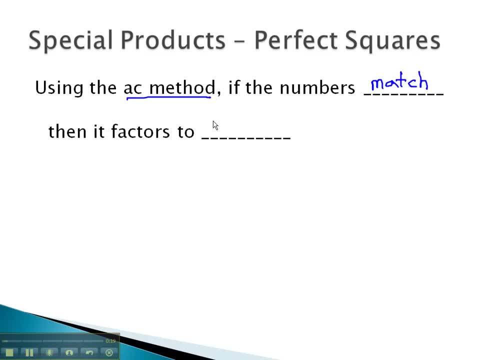 that will tell us that our solution, our polynomial, will factor to a perfect square, such as a plus b squared. Let's take a look at some examples where we find this relationship. In this problem, if we're using the AC method, we would be multiplying to 25 and adding to negative 10.. 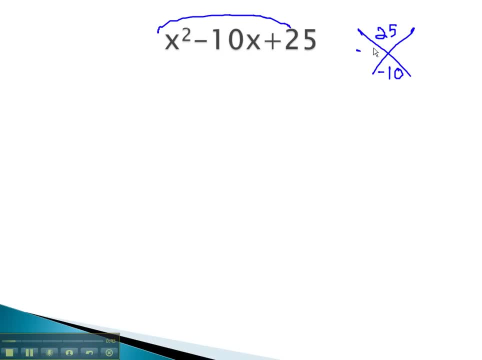 Try in a few combinations we find the answers we want are negative 5 times negative 5.. What becomes interesting about this combination is that the two numbers match. When that happens, we stop factoring by the AC method and jump straight to the perfect square that it factors to. 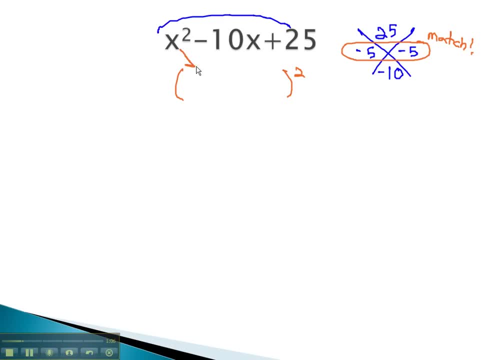 To factor a perfect square, we are going to take the square root of the first and last terms. The square root of x squared is x and the square root of 25 is 5.. The middle term tells us that a negative has to go in. 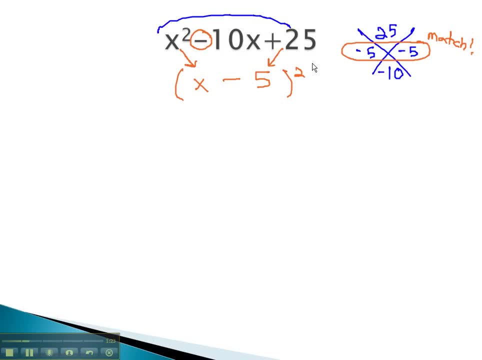 between the 5 and the x. After matching the sign from the middle term, we're now factored as x minus 5 squared. Let's take a look at another example, where we find the numbers from the AC method match, telling us we have a perfect square. 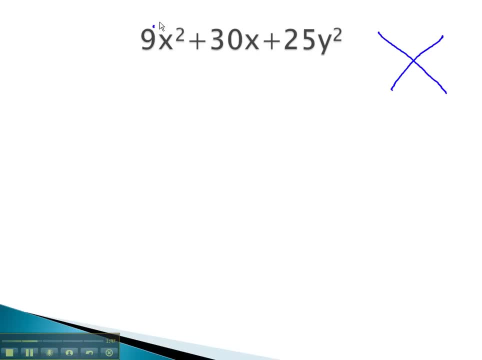 In this problem, using the AC method, we would be multiplying to 9 times 25, or 225, and adding to 30. These numbers are quite large so it might take a little guess and check in order to find the right combination of numbers. 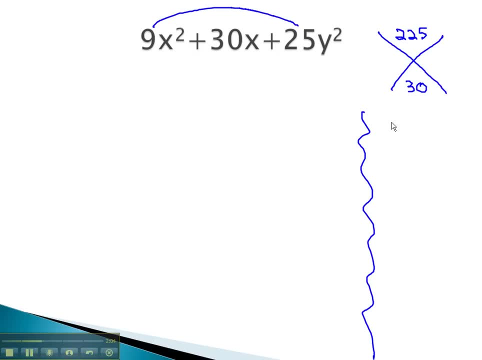 that multiply to 225. When, in doubt, start with 1 and count up 1 times 225 clearly will not add to 30.. 225's not divisible by 2, so next I try 3.. 3 times 75,, which does not add to 30 either.